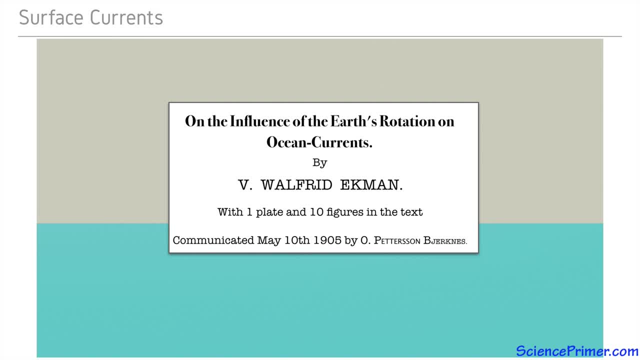 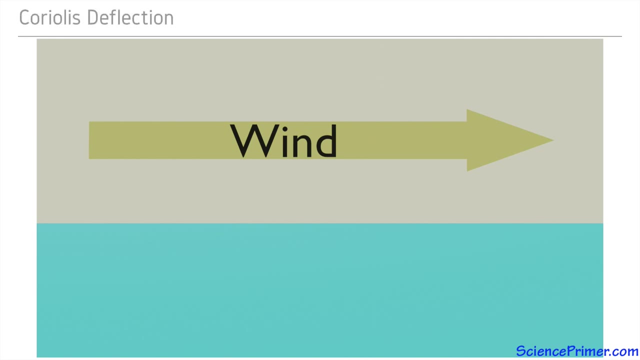 by the arctic explorer Fridtjof Nansen. While on an expedition, Nansen noticed that wind-blown sea ice did not move in the same direction as the wind. Instead, it moved 20 to 40 degrees to the right of the wind. He correctly speculated that this was due to the influence of Earth's rotation. 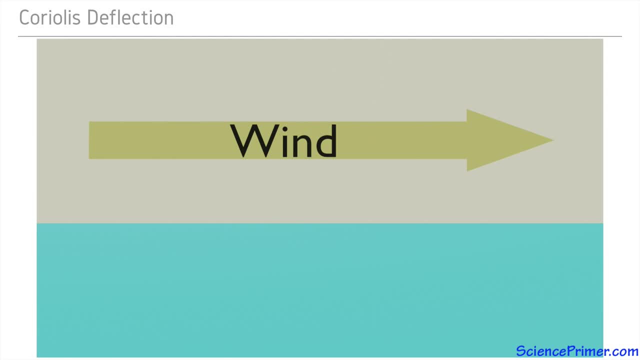 Ekman took Nansen's idea and built a mathematical model to explain it. Ekman's model treats water as a series of layers and water as a series of layers. Ekman's model is a series of layers which move independently of each other. As each layer moves, the energy from that motion can. 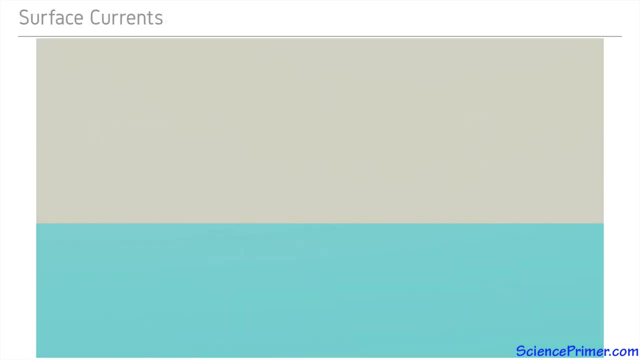 transfer from layer to layer. Consider a small vertical column of water that starts at the surface and extends towards the bottom. As energy moves from the surface to deeper layers, two things happen. First, because some energy is lost in each transfer to a deeper layer- water speed. 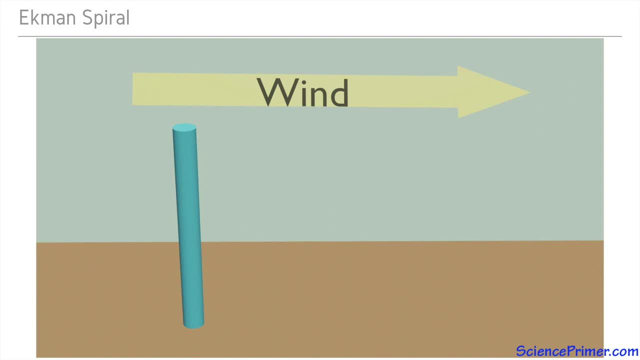 diminishes quickly with depth. Second, as the movement is transferred deeper, Coriolis effect creates a spiral pattern called an Ekman spiral. This creates a spiral pattern called an Ekman spiral. One result of this deflection pattern is that, at depth, a small amount of water is actually 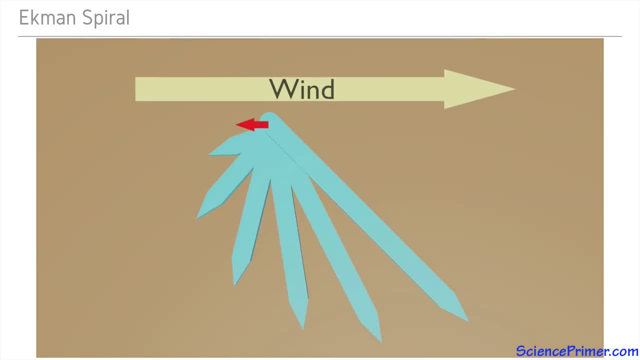 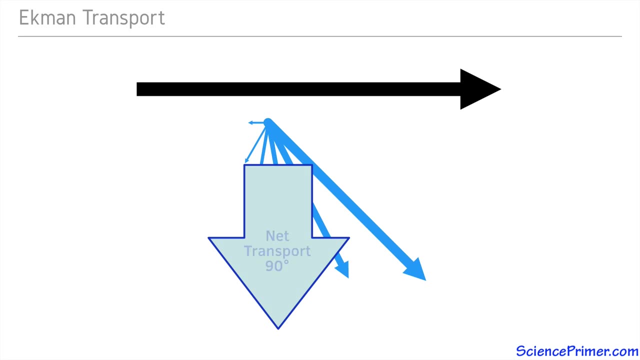 moving in the completely opposite direction than the wind that started the motion in the first place, Because water movement diminishes quickly with depth. Ekman showed that the net transfer of water is at a 90 degree angle to wind direction, Because this is all driven by the Coriolis effect. 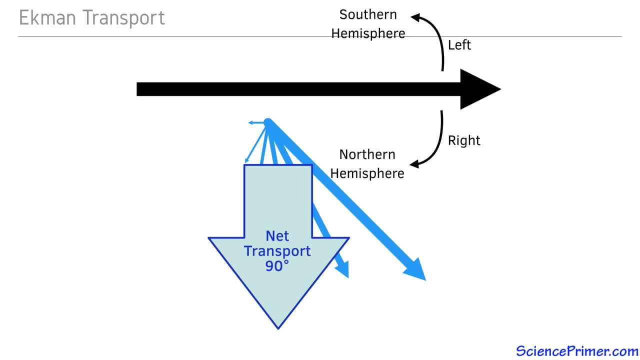 this deflection is 90 degrees to the right in the northern hemisphere and 90 degrees to the left in the southern hemisphere. This movement of water at right angles to the direction of the prevailing winds is called Ekman transport And, consistent with Nansen's observations, the water right at 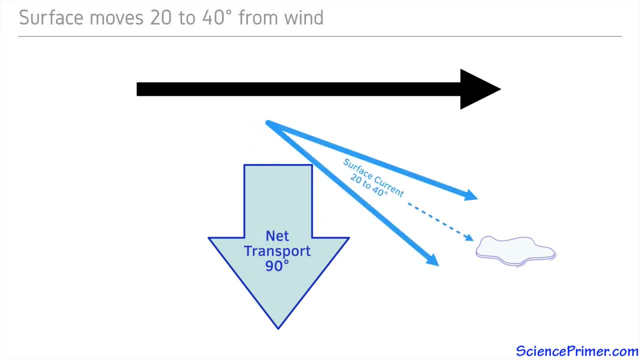 the surface moves 20 to 40 degrees to the right or left of the wind direction. This variability is driven by differences in how long and how consistently the wind blows. The dynamics of Ekman transport contribute to some important features in the ocean environment, including: 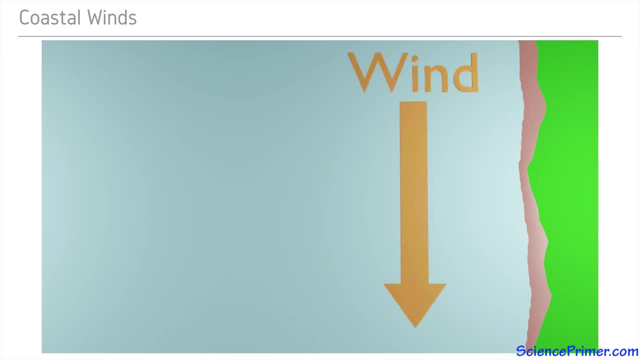 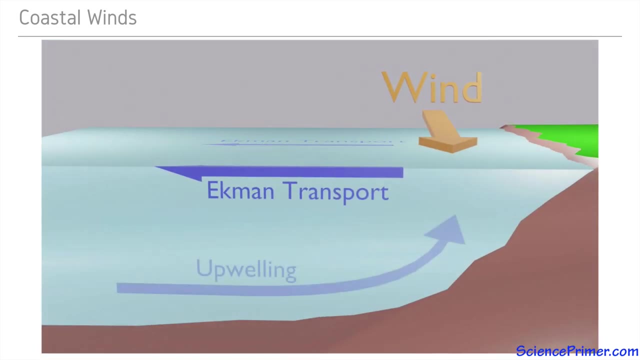 the fact that the wind is not pushing directly towards the coast. In coastal areas, where prevailing winds blow along the coast so that net water movement is offshore, the water pushed out to sea is replaced by deeper water, causing upwelling. The upwelling of this deeper water.